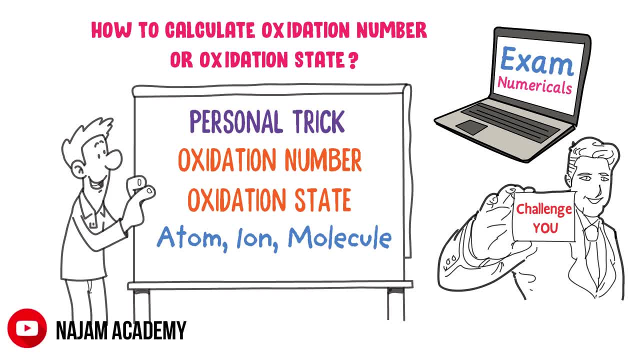 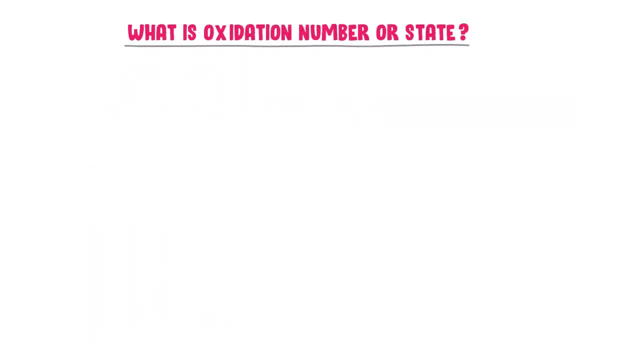 I will teach you exam-based numericals of oxidation number. Firstly, I will teach you that what is oxidation number or oxidation state? Well, the apparent charge on atom, ion or molecule is called oxidation number or oxidation state. For example, consider marketing sodium atom. 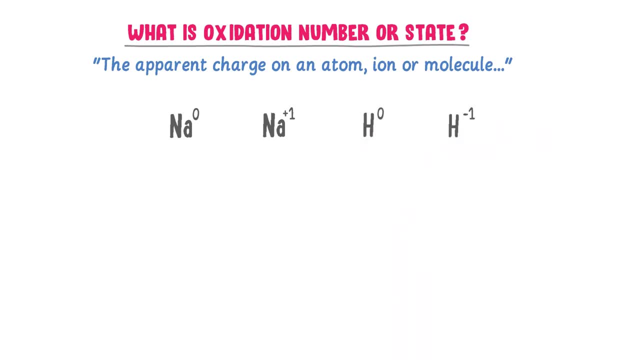 sodium ion, hydrogen atom & hydrogen ioncü. We know that sodium atom & hydrogen atom are neutral atoms. So the apparent charge on sodium atom is zero & the apparent charge on hydrogen ion and hydrogen ion is 0.. And what we counter-neutralize, lined up, is soda. be sure to. not to consider least topic. Make sure next discussion is on protocol. I shall use the next one, India, in a written guide. I have added much info in my blog & I will be providing links to the blog to you. If you want to check more detail, you can read it here, And please do not. 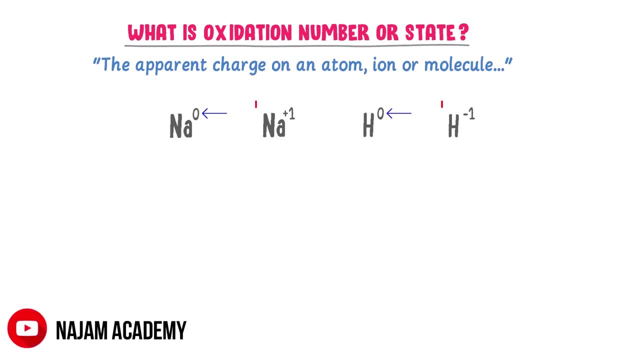 atom is also zero, while in the case of sodium ion and hydrogen ion, the apparent charge on sodium atom is positive: 1 and the apparent charge on hydrogen ion is negative: 1, so the oxidation state of sodium atom is 0. the oxidation state of sodium ion is positive: 1, the oxidation number of hydrogen atom is 0 and the 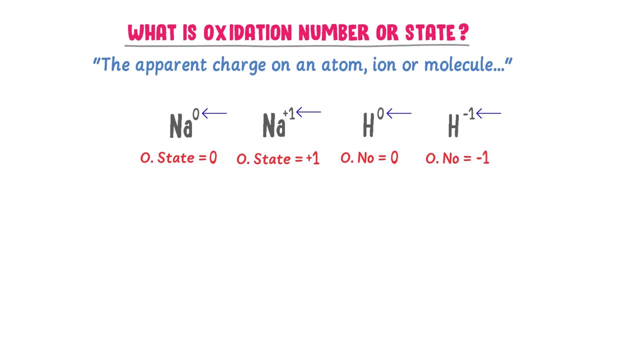 oxidation number of hydrogen ion is negative: 1. do not confuse if I say oxidation state or oxidation number, because they both are the same thing. similarly, consider iron atom, iron positive 2 ion and iron positive 3 ion. here the oxidation state of iron atom is zero. the oxidation state of this iron: 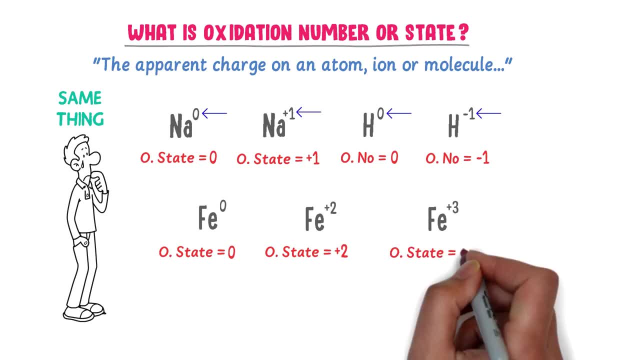 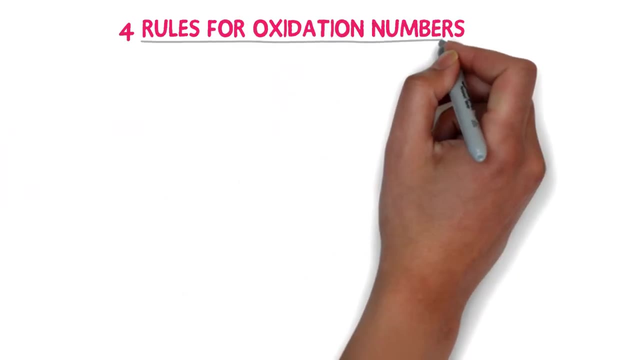 ion is positive 2 and the oxidation state of this iron ion is is positive 3.. Thus, remember that oxidation number or oxidation stat, is the apparent charge on an atom, molecule or ion. Now I will teach you only four simple rules for oxidation stat. 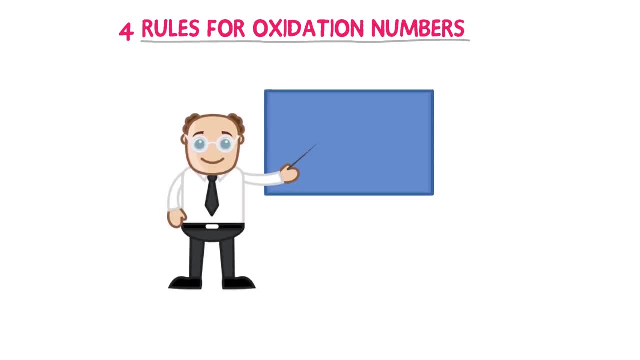 or oxidation number, and I am not going to teach you 10 or 20 boring rules which you often study in your school or college chemistry course. The first rule is that in free stat oxidation number is zero. For example, the oxidation number of sodium in free stat is zero, that of chlorine. 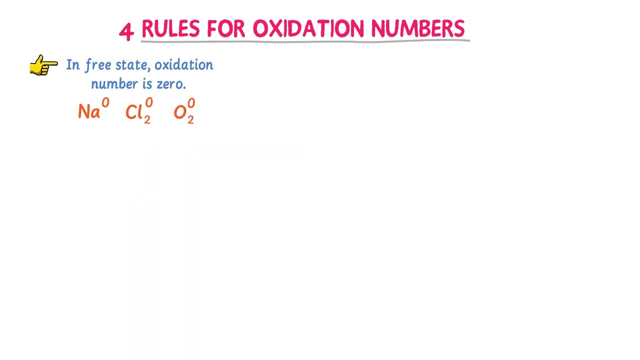 molecule is zero, that of oxygen molecule is zero and that of hydrogen molecule is also zero, While in the charge stat the oxidation number of an ion is the same as the charge on it. For example, the oxidation number of sodium ion is positive 1,. oxidation number of zinc ion is 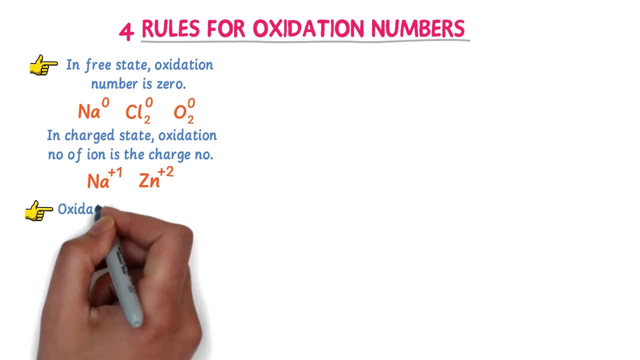 positive, 2, etc. Secondly, the oxidation number of hydrogen and its compound is positive 1 like an HCl, while the oxidation number of hydrogen and metal hydride is negative 1 like an sodium hydride. Thirdly, the oxidation number of halogen and its compound is negative 1 like hydrogen fluoride. Fourthly, 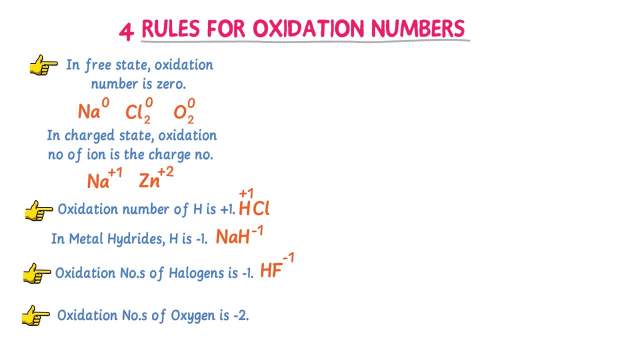 the oxidation number of oxygen and its compound is negative. 2, like an calcium oxide. Now, using these four rules, we can calculate the oxidation number of any atom, ion or molecule. Let me start from simple and easy examples. Find the oxidation number of magnesium and magnesium oxide. 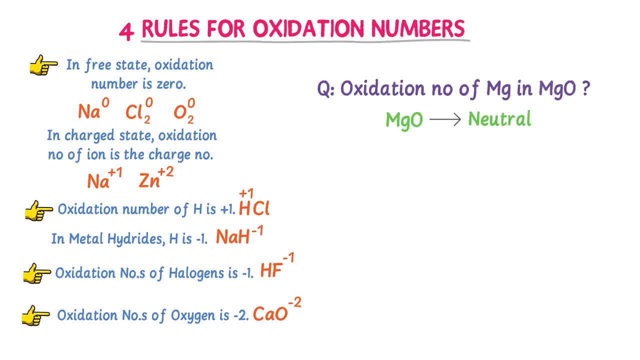 Well, magnesium oxide is a neutral ionic compound. The overall charge on it is zero, So the sum of all oxidation numbers must be equal to zero. I write: Mg plus O is equal to zero Because there is one atom of magnesium and one atom of oxygen and magnesium oxide. 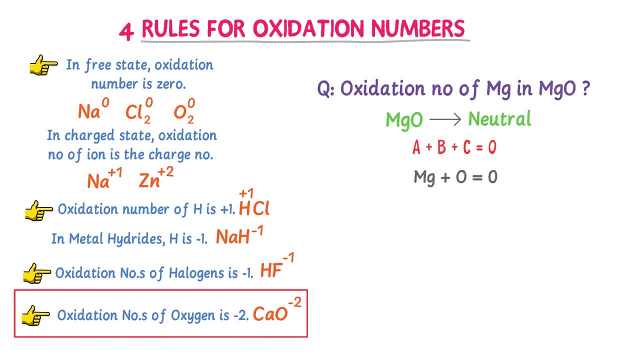 We know that the oxidation number of oxygen is negative two and its compound. So I put negative two instead of oxygen. Mg plus N to negative two is equal to zero, or Mg minus two is equal to zero or Mg is equal to positive two. So the oxidation number of magnesium and magnesium oxide is positive two and that of oxygen is 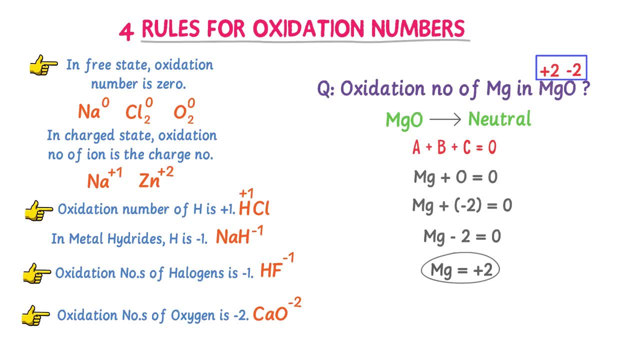 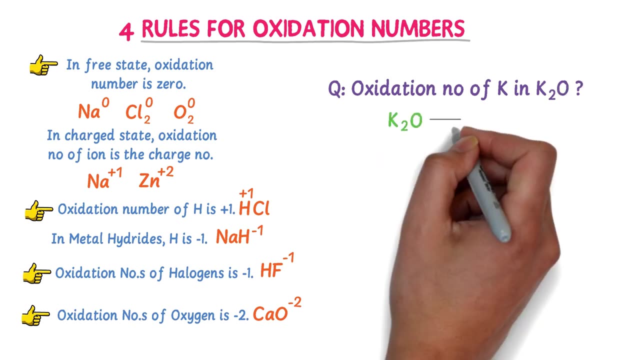 negative two, Also positive two and negative two cancel out. So we therefore say that magnesium oxide is a neutral ionic compound. Secondly, calculate the oxidation number of potassium and potassium oxide. Well, it is also a neutral ionic compound. The overall charge on potassium oxide is zero. 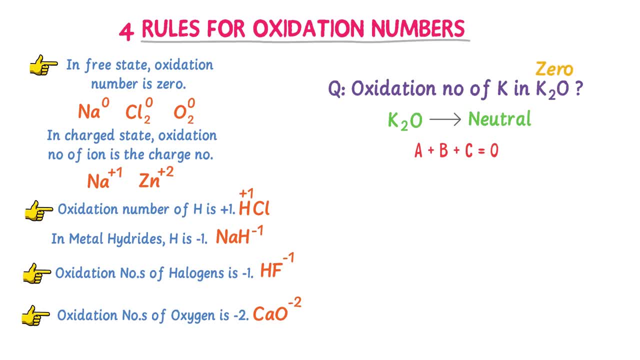 So the sum of all oxidation numbers must be equal to zero. I write: Mg plus O is equal to zero, Because there is one atom of magnesium oxide and one atom of oxygen present in potassium oxide. I write: Mg plus O is equal to zero. 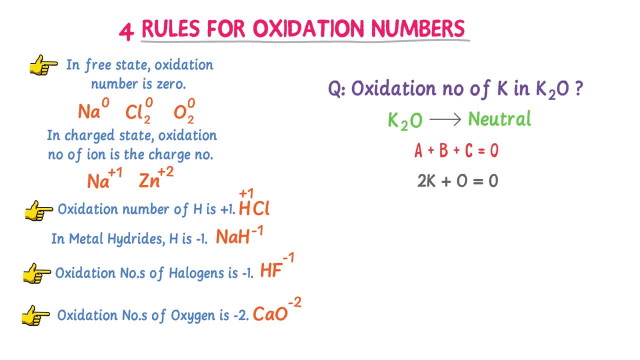 I write, Mg plus O is equal to zero. Here I write Mg because there are two atoms of potassium and one atom of oxygen present in potassium oxide. The oxidation number of oxygen is negative two and its compound. So Mg plus N to negative two is equal to zero, or Mg is equal to two. 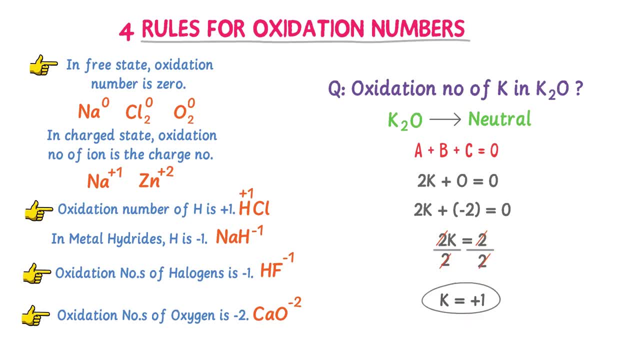 Dividing both sides by two, We get K is equal to positive one. Thus the oxidation state or oxidation number of potassium is positive one and that of oxygen is negative two. Remember that oxidation number of one potassium atom is positive one and two potassium atom. 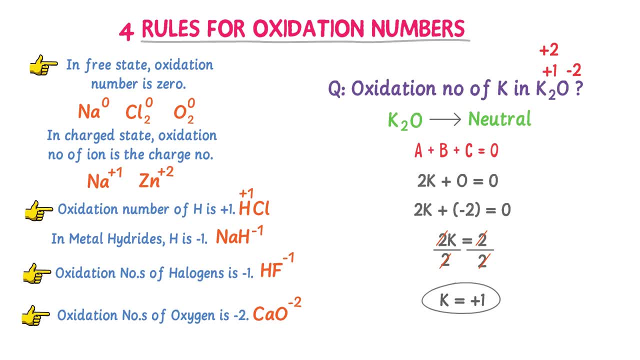 is positive two, So positive two and negative two. cancel out and overall we get zero charge on potassium oxide. Now let me take you to the medium level. Find the oxidation number of nitrogen and NH3.. Well, it is a neutral molecule. The overall charge on it is zero. 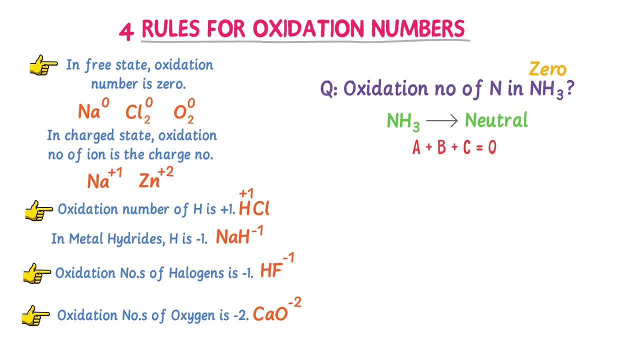 So the sum of all the oxidation number must be equal to zero. I write: N plus 3H is equal to zero. Here there are one atom of nitrogen and three atoms of hydrogen present in ammonia, NH3. We know that the oxidation number of hydrogen and its compound is positive one. 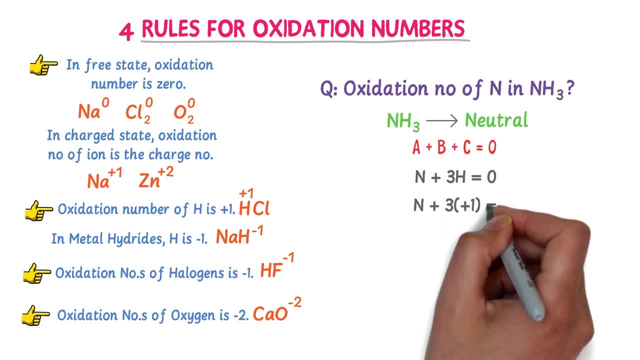 So it is positive one. Find the oxidation number of nitrogen and NH3. Well, it is a neutral molecule. So I write N plus 3N to positive. one is equal to zero. Rn plus 3 is equal to zero. Rn is equal to negative three. 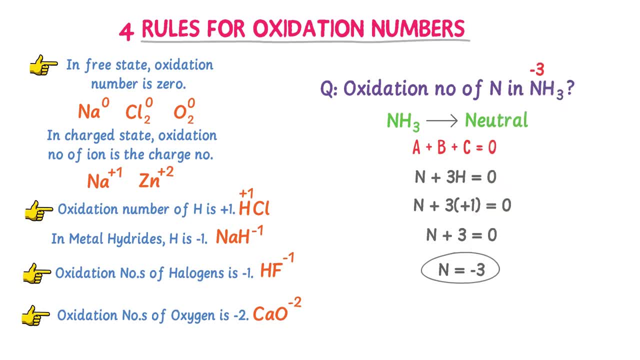 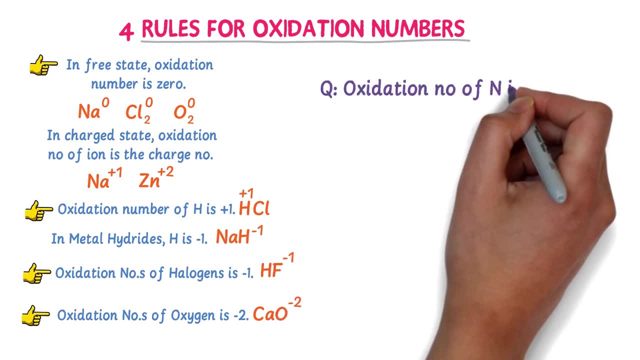 So the oxidation number of nitrogen is negative three, and that of hydrogen is positive one. and ammonia, NH3.. Secondly, find the oxidation number of nitrogen and nitrogen dioxide ion. Well, it is an ion, The overall charge on it is negative one. So the sum of all the oxidation numbers must be equal to negative one. 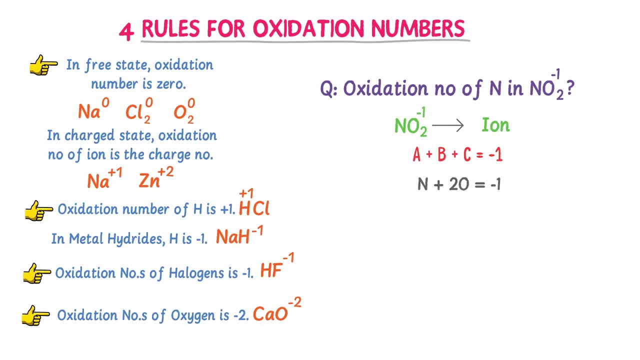 I write, N plus 2O is equal to negative one. There is one atom of nitrogen and two atoms of oxygen present in nitrogen dioxide ion and the overall charge on it is negative one. We know that the oxidation state of oxygen and its compound is negative two. 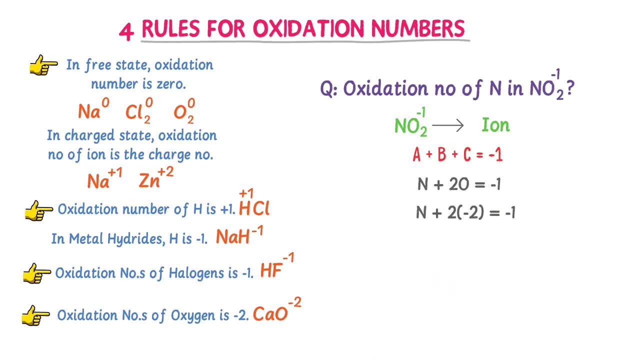 So I write N plus 2N to negative two. So I write N plus 2N to negative two is equal to negative one. Rn minus 4 is equal to negative one. Rn is equal to positive three. Thus the oxidation state or oxidation number of nitrogen is positive three and that of 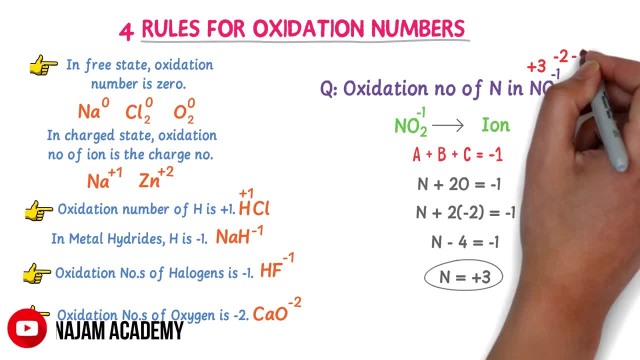 single oxygen is negative two, While there are two atoms of oxygen are present. So negative two plus negative two is equal to negative four. Therefore positive three, negative four is equal to negative four equal to negative 1 and overall the charge on nitrogen dioxide ion is negative 1.. 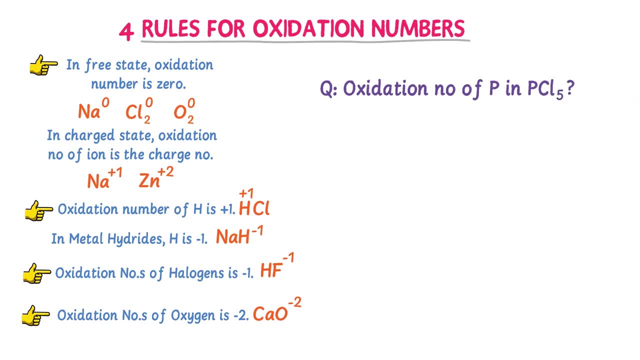 Thirdly, find the oxidation number of phosphorus in PCl5.. Well, it is a neutral molecule. The overall charge on it is zero, So the sum of all the oxidation numbers must be equal to zero. I write: p plus 5. Cl is equal to zero, because there is one atom of phosphorus and five atoms. 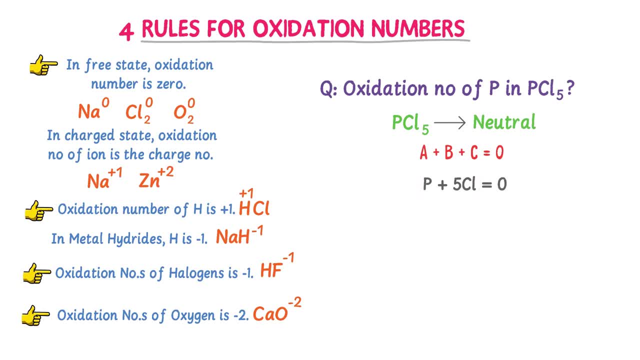 of chlorine present in PCL5.. We know that the oxidation number of halogens and their compounds is negative, 1.. So p plus 5 into negative 1 is equal to zero. Our p minus 5 is equal to zero. Our p is equal to positive 5.. 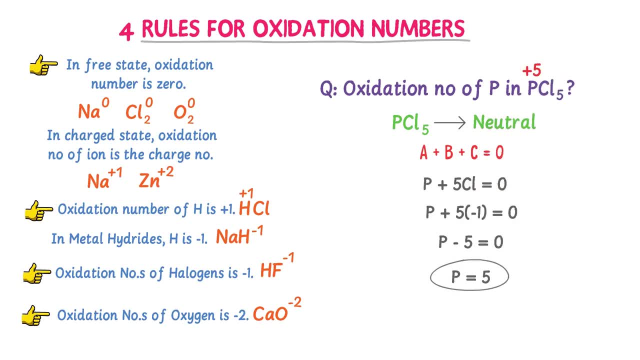 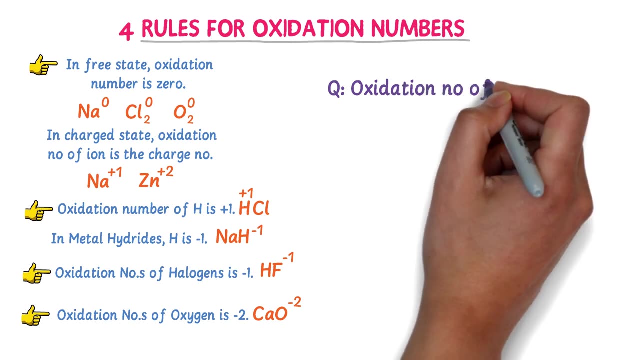 Thus the oxidation number of phosphorus is positive 5 and that of 1 chlorine is negative 1, while that of 5 chlorine is negative 5.. Now let me teach you some exam based questions of oxidation numbers. Find the oxidation state of sulfur and H2SO4 are sulfuric acid. 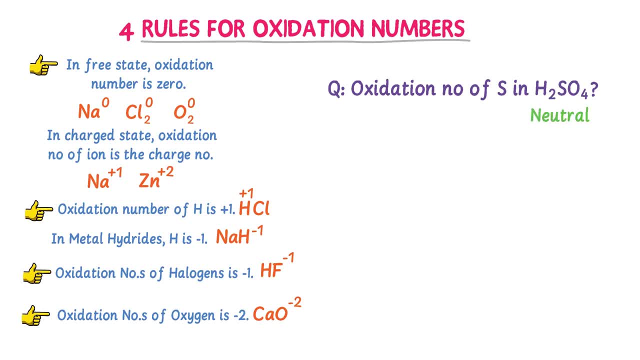 Well, it is a neutral molecule. the overall charge on it is zero, So the sum of all oxidation numbers must be equal to zero. I write: 2H plus S plus 4O is equal to zero because there are two atoms of hydrogen: one. 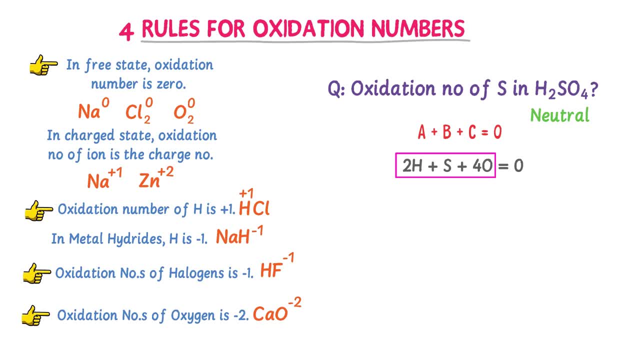 atom of sulfur and four atoms of oxygen are present and H2SO4.. We are asked to find the oxidation number of sulfur, hence it is our subject. We know that the oxidation number of hydrogen and its compound is positive: 1 and that of 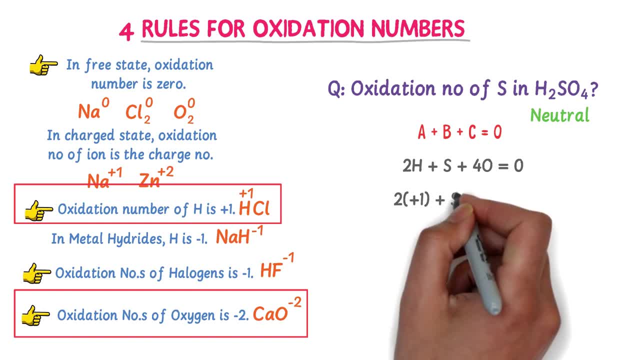 oxygen is negative 2.. So I get 2 into positive, 1 plus S plus 4 into negative. 2 is equal to zero. R2 plus S minus 8 is equal to zero R. S is equal to positive six, So the oxidation number of sulfur is positive six. 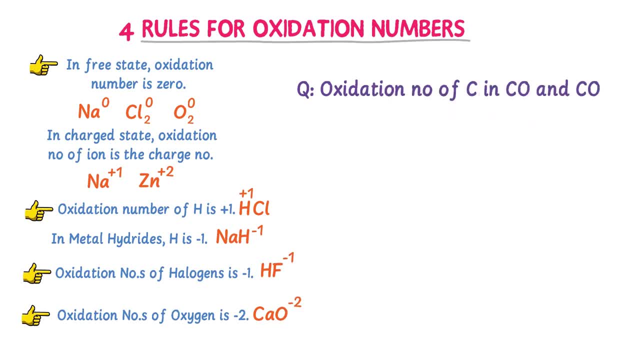 Secondly, find the oxidation number of carbon and carbon monoxide and carbon dioxide. Well, we know that monoxide and carbon dioxide are neutral molecules. So in case of carbon monoxide, I write: carbon plus oxygen is equal to zero. We know that the oxidation state of oxygen is negative, 2. So 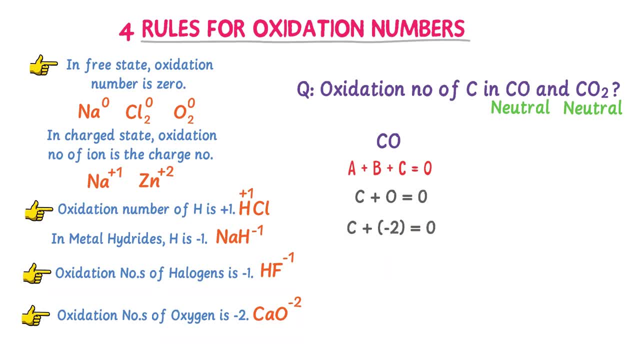 carbon plus N2- negative 2 is equal to zero, or carbon minus 2 is equal to zero, or carbon is equal to positive 2. While in case of carbon dioxide I write carbon plus 2 O is equal to zero. The oxidation state of oxygen is negative 2.. So carbon plus 2 N2- negative 2 is equal to zero. 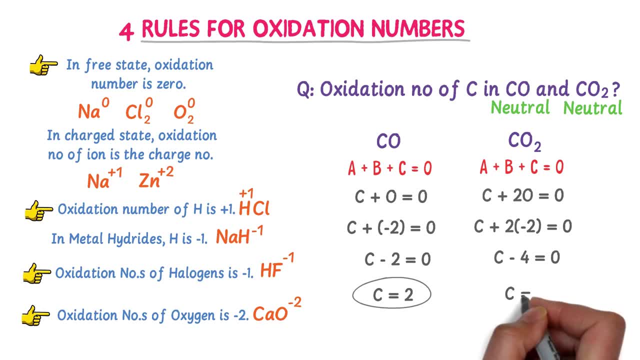 or carbon minus 4 is equal to zero or carbon is equal to positive 4.. Thus, the oxidation number of carbon and carbon monoxide is positive 2 and the oxidation number of carbon and carbon dioxide is positive 4.. From this example, we also learn that oxidation number of the same 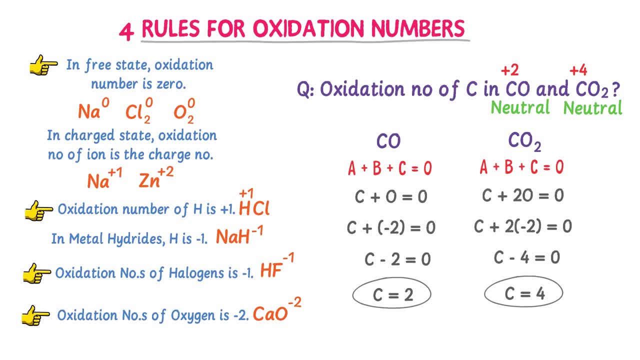 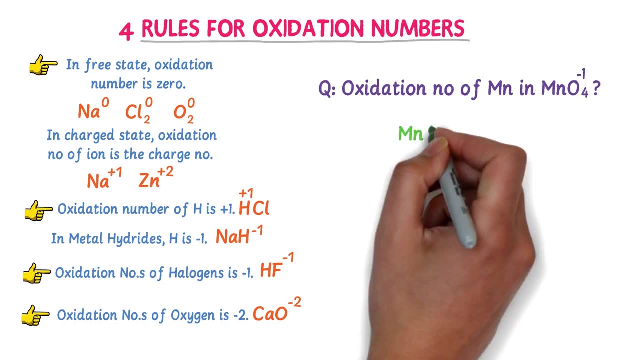 atom like carbon can be different in different substances. Thirdly, find the oxidation number of manganese and manganese oxide ion. Well, it is an ion. The overall charge is negative 1. So the sum of all the oxidation number must be equal to negative 1. I write Mn plus 4 O. 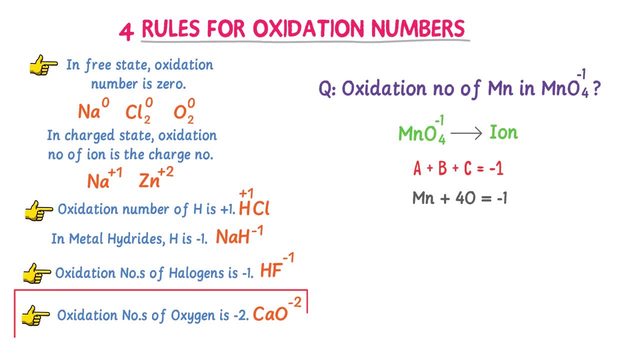 is equal to negative. 1. We know that the oxidation number of oxygen is negative, 2. So Mn plus 4, N2, negative 2 is equal to negative. 1 or Mn minus 8 is equal to negative. 1 or Mn is equal to positive.